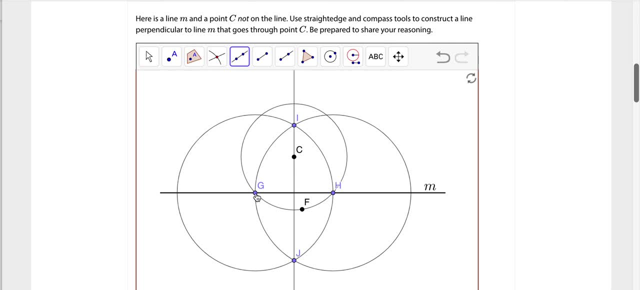 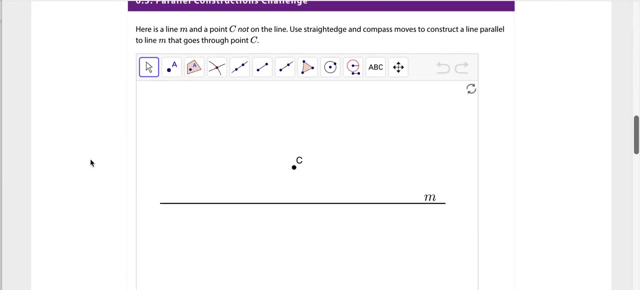 this is the set of all points equidistant from the two endpoints, in this case G and H. Alright, so that's the perpendicular line. Let's move on to the parallel one. Now it might feel kind of counterintuitive, but to create a parallel line we are going to first. 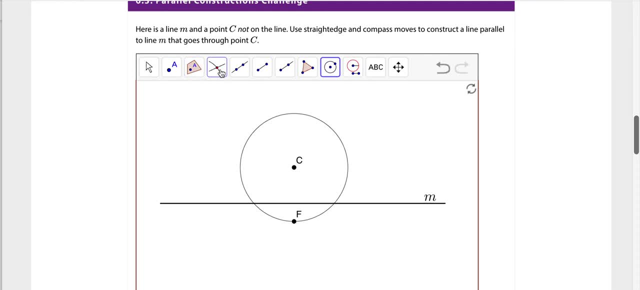 create a perpendicular line. So I'll do the exact same thing I did last time: Create the circle that intersects with line M. get those two endpoints, create the perpendicular bisector That's going to get me a line. So I'm going to create a line perpendicular to M that passes through point C. Now why? 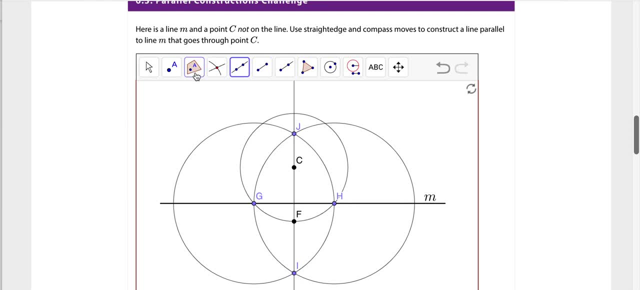 in the world would I want to create a perpendicular line? when it was asking me to create the line parallel to M. Well, if you create a line that's perpendicular to this new line, by default it will be parallel to line M. So, basically, I'm going to repeat that same process. 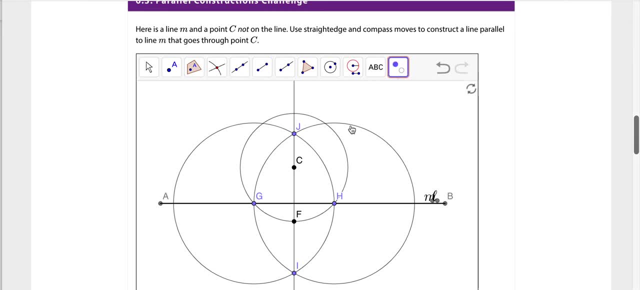 all over again. Now, just to kind of show you more simply what's happening, I'm going to hide all of the circles and points that I've made so far, so that we just have the line M that was given to us, the point C that was given to us and my new perpendicular line. 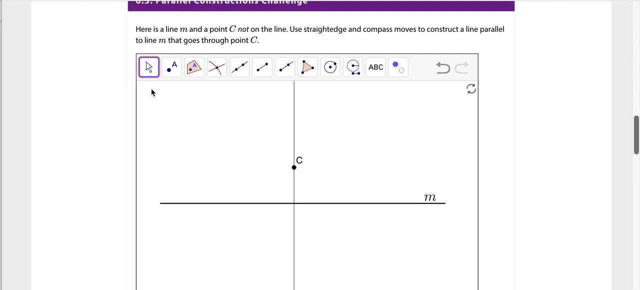 that we just did in the last problem. So what we're going to do now is we're going to try to kind of repeat the process where we're going to make a line perpendicular to this new line that I've added- And if you can visualize it, that will be parallel to line M- To make. 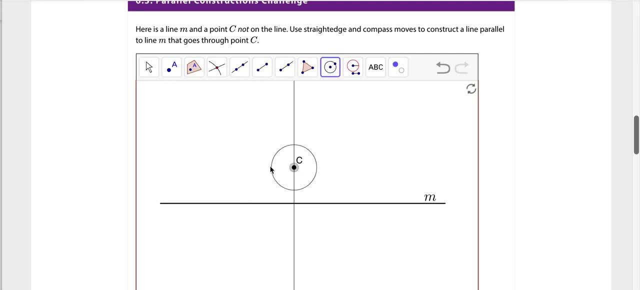 a line perpendicular to this new line. we're going to go through point C. we'll do the same starting move we did the last time: Make a circle, find the two intersection points with the line. Now, this time, C was on the line to begin with, so we're just finding. 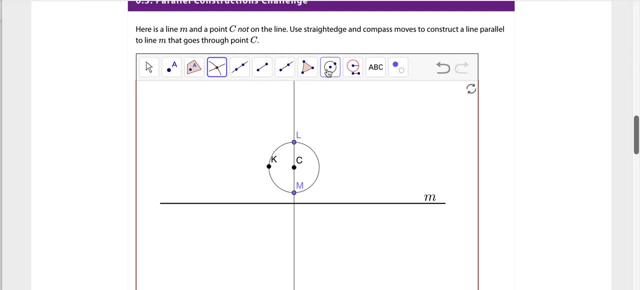 two other end points along that line And you actually could have used the first circle we used before, but I'm just making a smaller one so I can see this a little bit separately. And then, if you kind of turn your head sideways, try to visualize repeating the process of 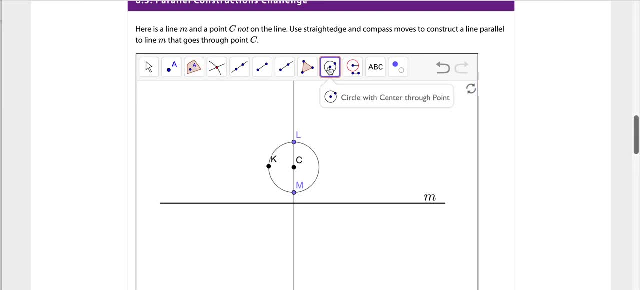 L, M. So instead of making the circles kind of side-by-side, they'll be stacked on top of each other like this. But that's that sideways perpendicular bisector to what we just did before. I find the two intersection points and guess what? This line that goes through.